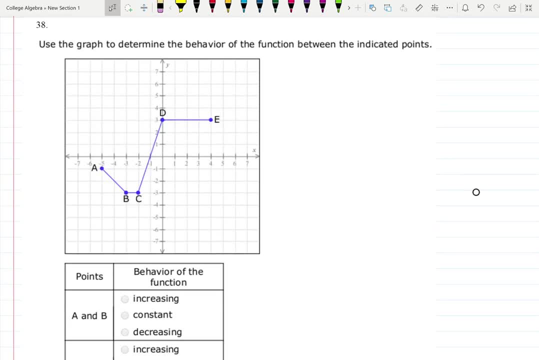 the mountain and when you're hiking the mountain it's either hard to hike because it's going up, it's easy to hang because it's going down, or maybe it's just the flat hike so you don't feel like up and down at all, Just the valley right. So if you put your pencil on the graph, 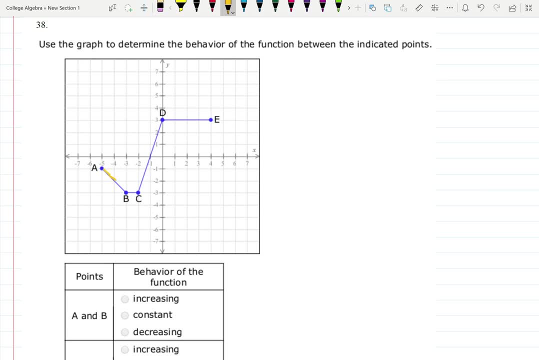 of the function and your pencil is sliding down. so you're going down. when you hike, it's sliding down. this is where the function is decreasing. If you put a pencil and your pencil is going up, that's where the function is increasing. if your pencil is going horizontally, that's like a floor. 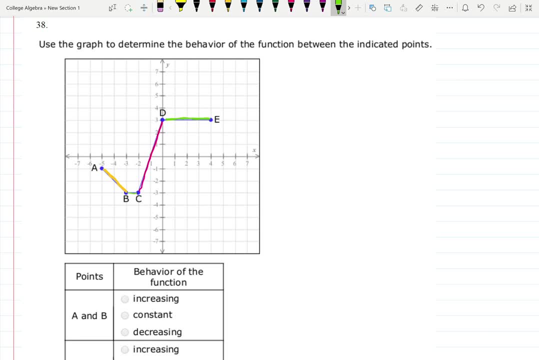 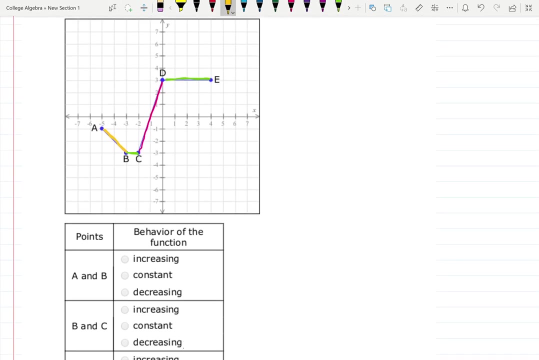 so the floor of the room is not increasing, not decreasing. it's flat, so that's where the hike is flat. that's why the function is constant. well, let's now answer the questions. they ask what happens between points a and b in orange color, or yellow, between a and b. my pencil was sliding down, so here the function is decreasing. 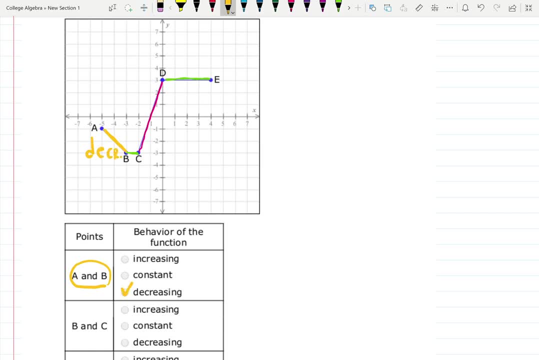 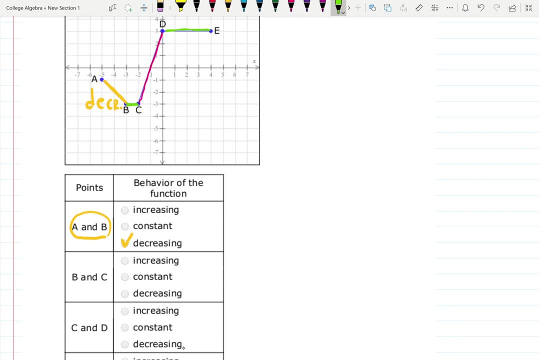 it makes sense, simple as that, no tricks at all. what is happening between b and c, between b and c? i put a pencil here and the pencil did not go up and did not go down. so it means the function there is constant and you even can write down the function equation if the constant is minus three. 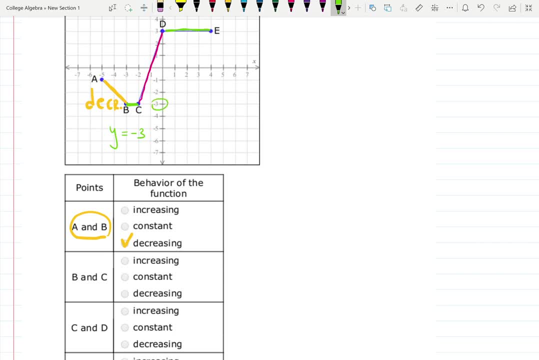 because it's fixed at the height minus three. that's the next really extra information. you don't actually have to know it for this topic, but in the future you will get how all of this connected is connected to you together. so it's constant here, not decreasing and not increasing. 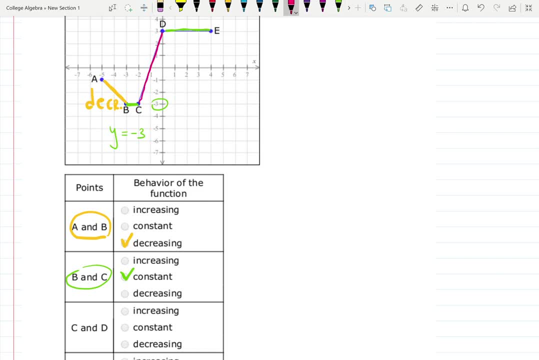 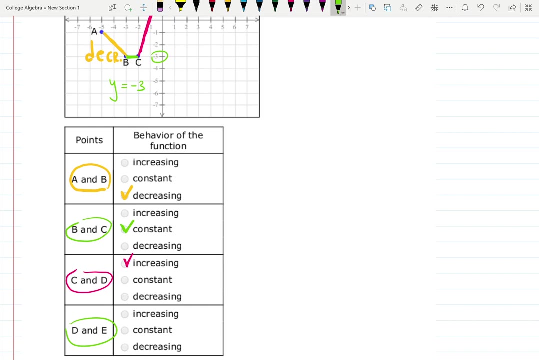 lastly, between c and d. well, it's not the last question, but still between c and d. my pencil was going up. i can even put the arrow like this, up, then it's increasing. it's going to be a hard hike, so you have to climb up. finally, between d and e. again, it was flat, remember. look at it. 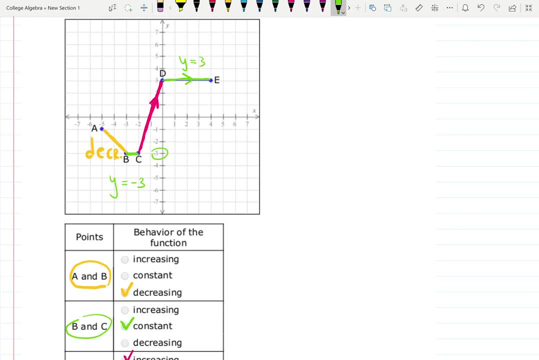 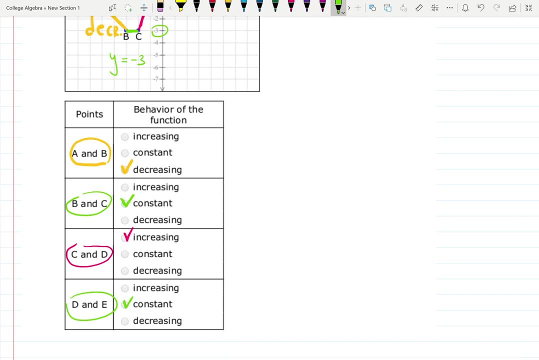 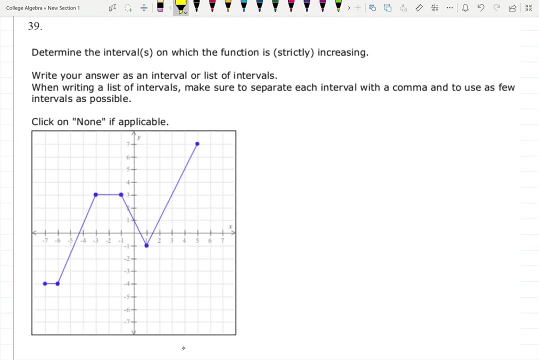 between d and e. it's flat, and it's y equals three. the height of this line is: so that's a constant equation of a constant line. i even show it to you now. you know now what if they ask you those funny questions about strictly increasing, strictly decreasing? 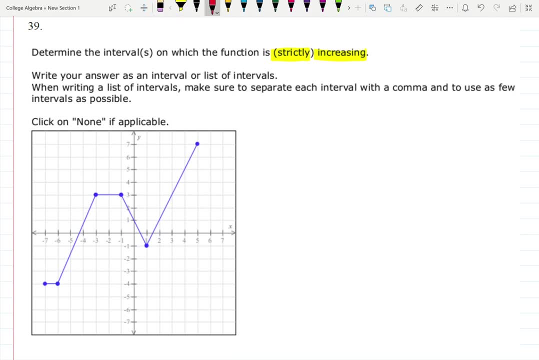 and so on. you have to figure out by yourself and use internet interval notation, not internet interval notation, to write the answer interval notation. so let's see that there's no a, b and c here anymore. so let's see that there's no a, b and c here anymore. so let's see that there's no a, b and c here anymore. 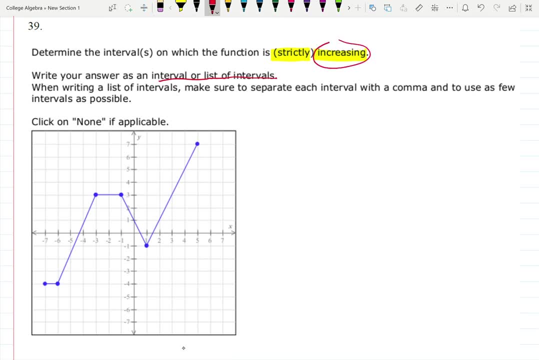 they ask me where the function is increasing. strictly increasing means you don't include the end points, so the interval will have parentheses, like this again. let me think where. what is going on with the function? i'll put pencil on the graph and start walking- walking horizontally, now, that's flat. walking up: yeah, that seems like increasing. 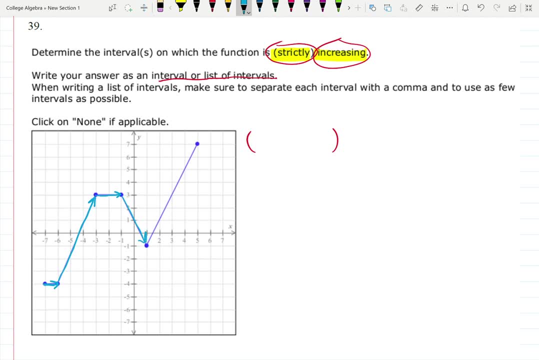 horizontally: no, that's constant going down, there's decreasing. going up, yes, that's increasing. so that's how you know. i will just point out to myself every time my pencil was increasing on the graph like: so that is exactly where i should indicate that the function is strictly increasing. 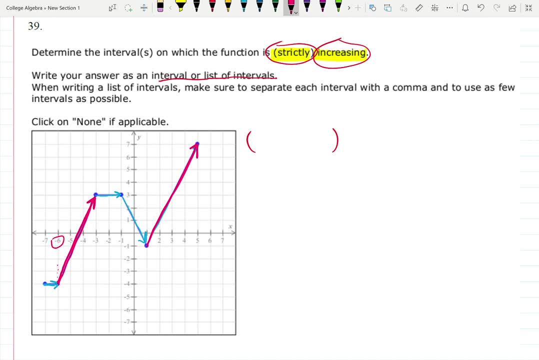 this happens from minus six. how do i know? i'll just put it up up like this. and then stopped happening at negative three. so from minus six to minus three, without including end points, because it's strictly increasing, the function is increasing comma, and it also happens from one and up until five. so from one to five, without including. 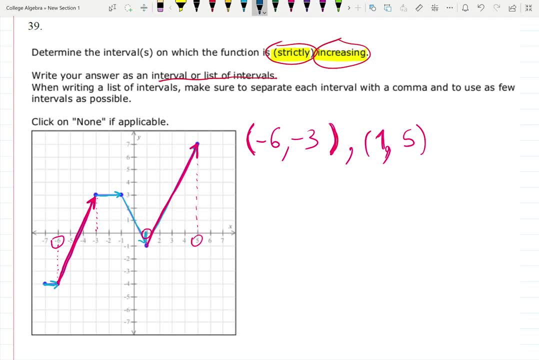 the end points. it's also increasing. would you like to write down where the function is decreasing really fast? stop the video and do it by yourself and then compare with my hands, decreasing from negative one to one. so i will write down like this: decreasing from negative one to one. 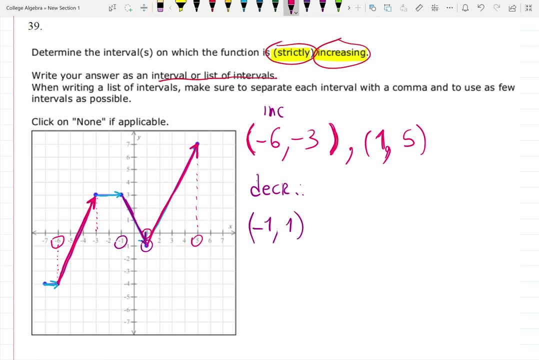 we were answering questions about increasing, increasing and then also constant. let's answer the question about constant. constant happened at from negative seven- it's over here- from negative seven to negative six comma. then it was also constant from negative three to negative one, from negative three to negative one comma, and oh, that's all. so now, as you can see, all three.